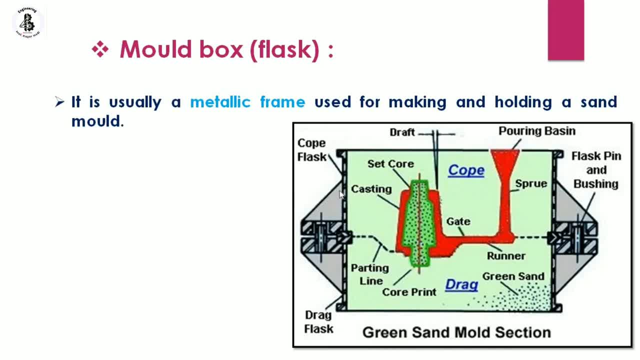 flask. so basically that will be dividing into two categories: the upper part that will be known as a cope, so that cope, which will be fixed with a cop flask, and lower part that will be drag, so drag. it will be connected with a drag flask and into that mold box there will be the some different terminologies we will discussing on. 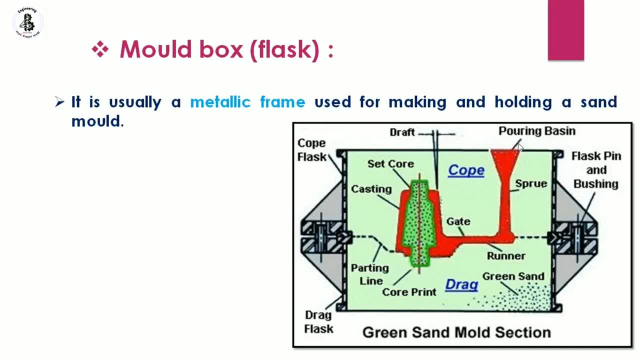 to later. but just you can see, wearing business sprue runner, get castings, set the course if the core print is being required, so core prints, so that all category or you can say cop, flask and drag flash, which will be corrected with a flash pin and bushing, so that whole the assembly of 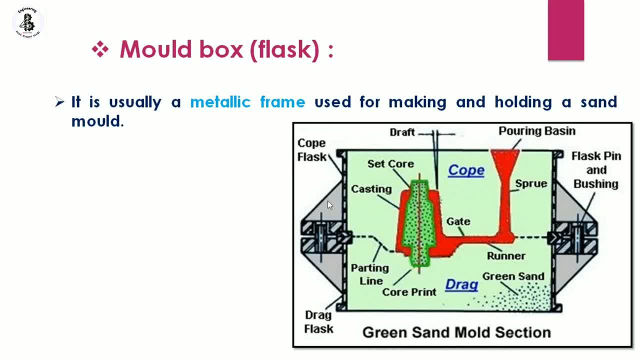 cope and drag that will be known as a mold box, the next so the mold box, which will be two types: the upper part that will be known as a cup and a lower part that will be called to be a drag. so second, one parting line or you can say parting surface, so just you can see. 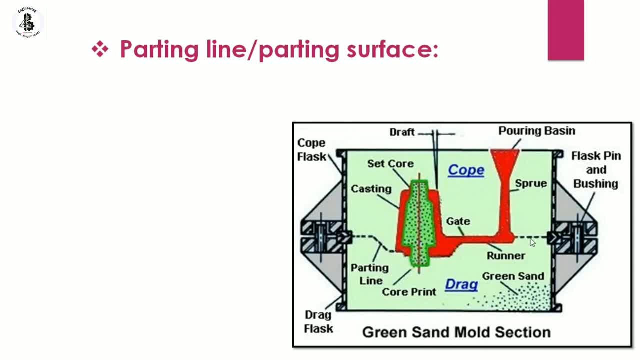 this dotted line which will be separating both the upper part and lower part, so on to the upper part, that will be the cop and lower part, that will be the drag. so this parting line that will be. you can see that in simple way. it will be a. 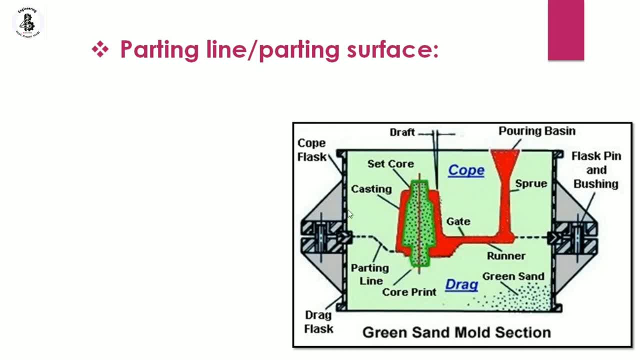 separating line of cop and drag. so it is the zone of separation between cop and drag. portion of a mold into a sand casting process, then sprue. so just you can see the sprue, that one. so after the pouring basin it will be connected with the sprue. to sprue is nothing, but it will be a vertical passage through which. 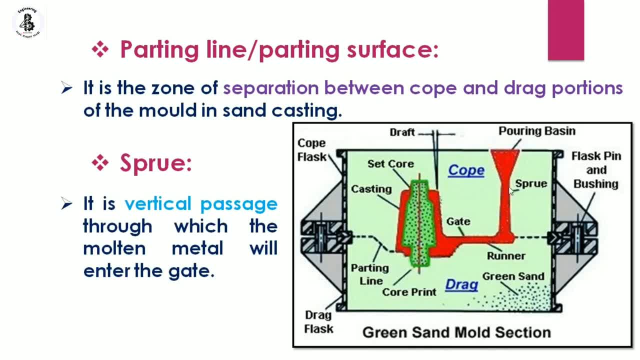 the molten metal it will be entering into the gate said initially that will be the pouring basin. so all the molten form of the matter that will be collecting into the pouring basin and this section so you can say vertical passage. so that will be providing the passage. 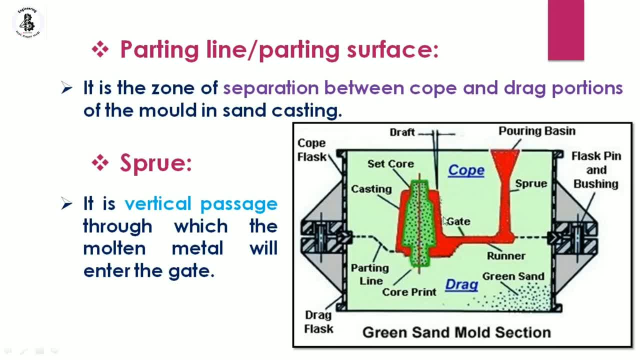 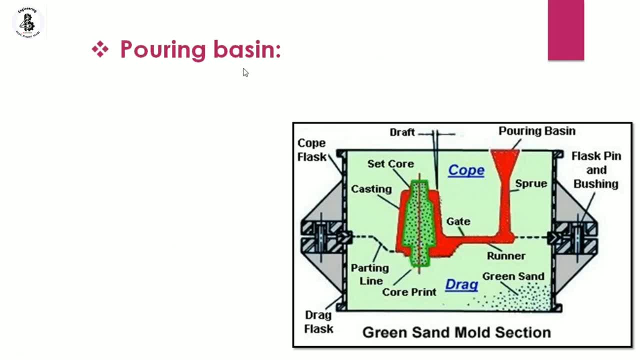 for filling of a cavity. so starting vertical passage that will be known to be a sprue. the next pouring basin, so that upper part, it will be known as a pouring basin, so the enlarged portion of the sprue at the top, so which molten matter is to be poured, so you can easily controlling the flow of the molten. 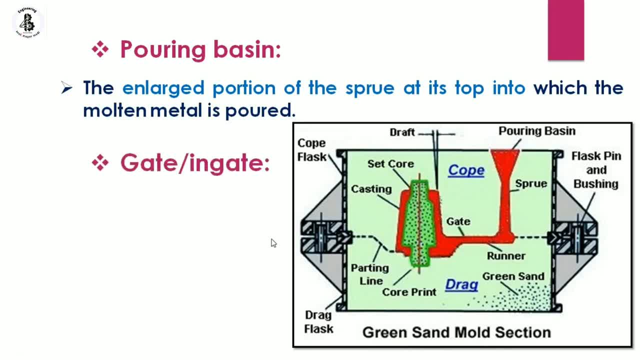 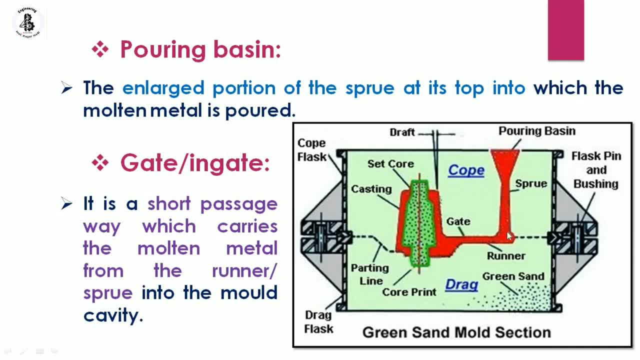 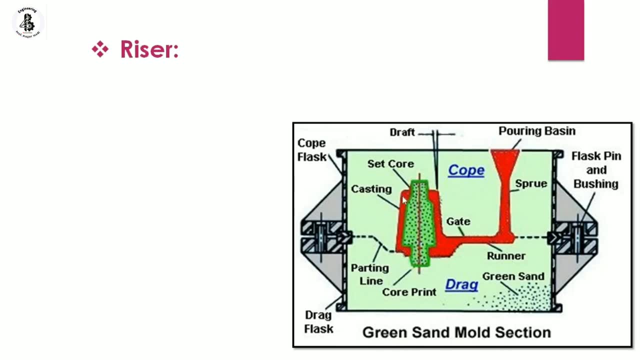 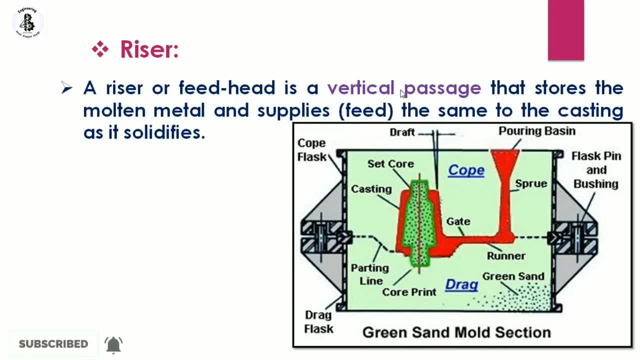 or you can say riser, that will be half during the solidification process. so that will be the requirement of the some another molten form of the materials. so by this riser it will be collecting of the molten form of the metals. so according to that requirements of the solidifications. 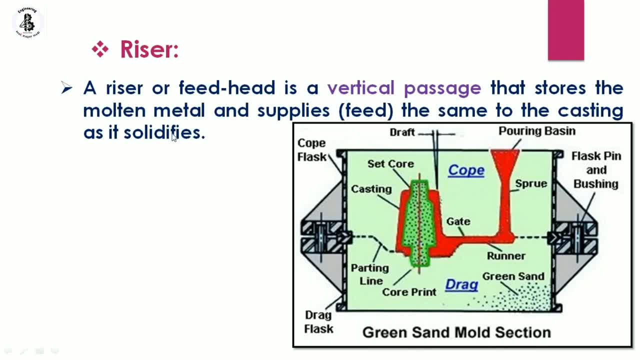 so by this solidifications of the castings, that additional materials it will be providing by the riser and riser it will be also give the hundred percent ensurement regarding to the filling of the cavity and that will be also help for escaping the airs which would be present. or you can say: